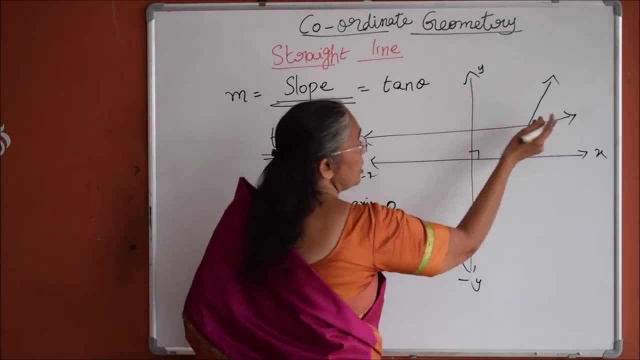 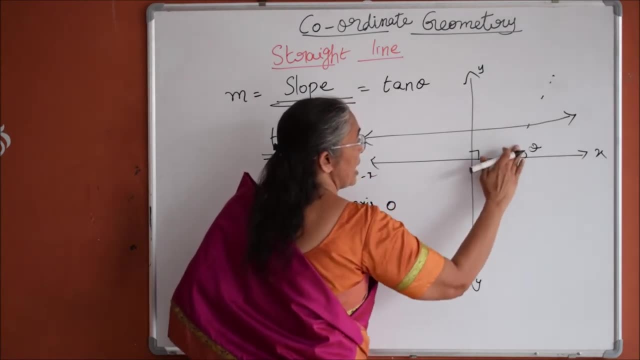 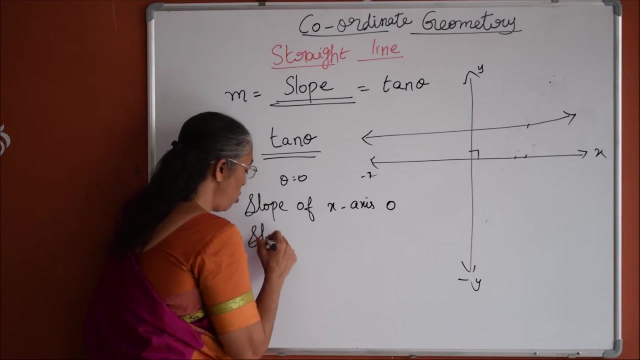 x axis also, because now with this also the line is: this is a line, So this line is not making any angle with the positive direction of x axis. So the angle made by this line with x axis is 0.. So slope of x axis and slope of a line parallel to x axis. slope of a line. 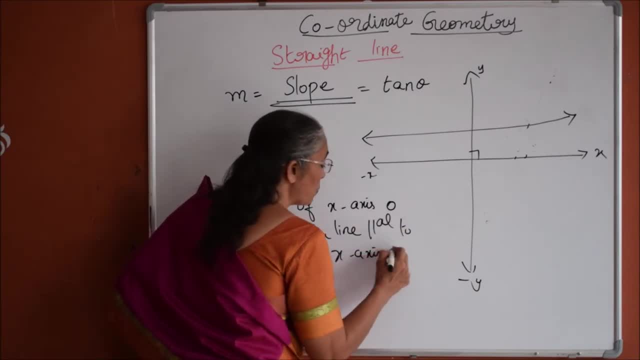 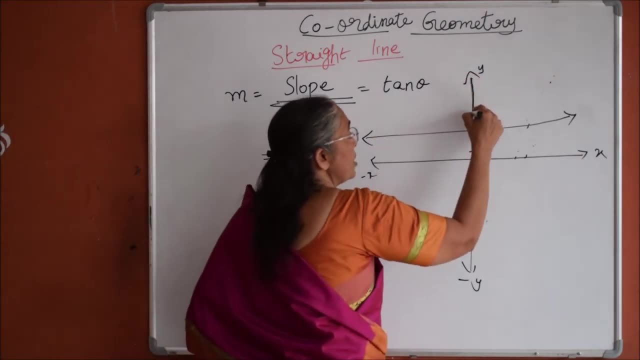 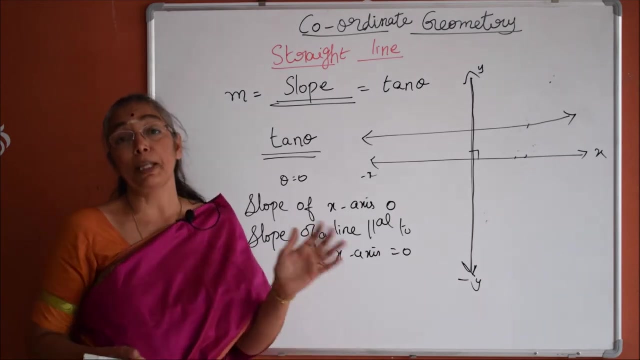 parallel to x axis. both are 0.. Now, similarly, what can be the slope of y, slope of a y axis, Now slope of this line. so what is the definition of slope? The tan of angle, tan of the inclination made by the straight line with the positive direction of x axis. 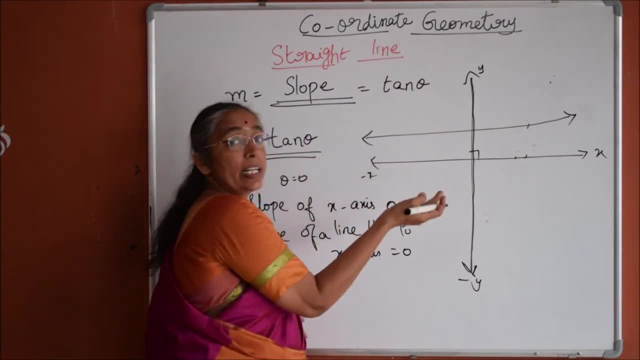 So now? so what is the definition of slope? The tan of angle, tan of the inclination made by the straight line with the positive direction of x axis, is 0.. Now, slope of y axis will make an angle of 90 degrees with the x axis, So tan 90, tan 90 is infinity, So slope similarly. 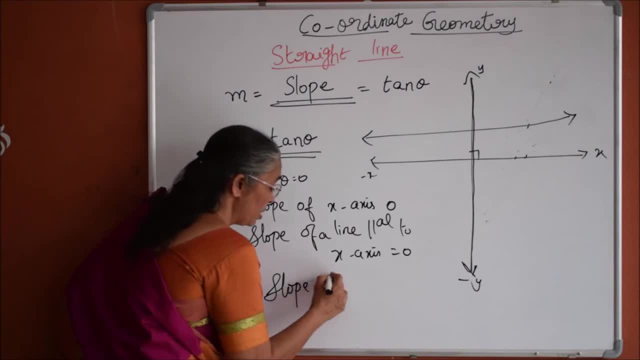 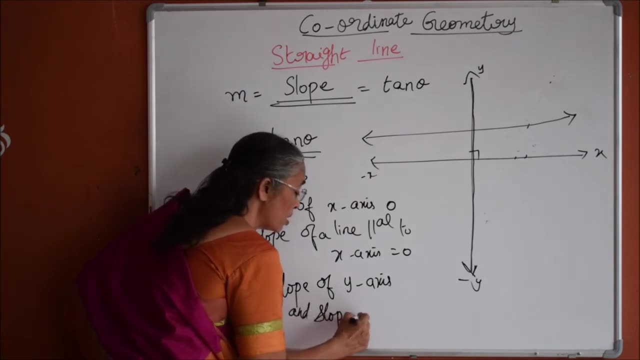 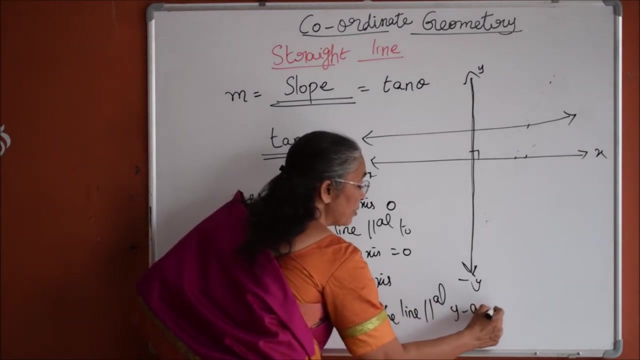 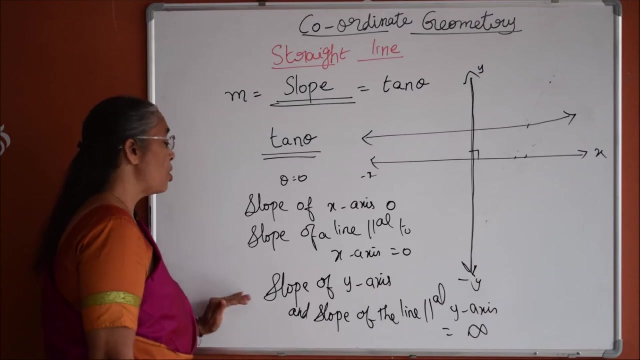 even for the line parallel to y axis. slope of y axis and slope of the line parallel to y axis. slope of the line parallel to y axis: both are infinity Clear children. Slope of x axis and slope of a line parallel to x axis is 0.. Slope of y axis and slope of the line. 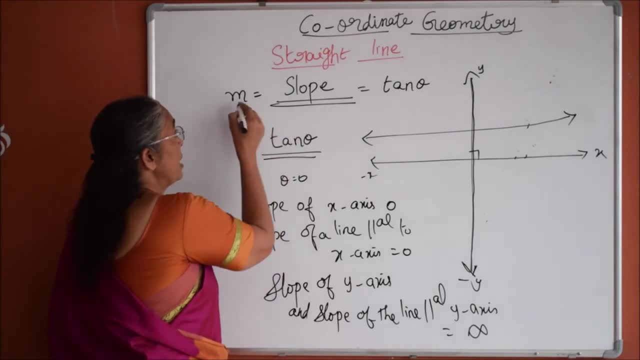 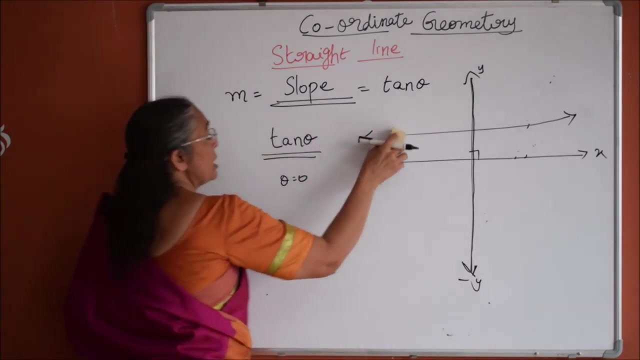 parallel to y axis is infinity. So main, basically tan theta, is the slope. that is the one form. Now, if two points are given, how to get the slope of the line, Okay, So this is based on the angle we got Now instead of angle. suppose two points are given. Okay, So this: 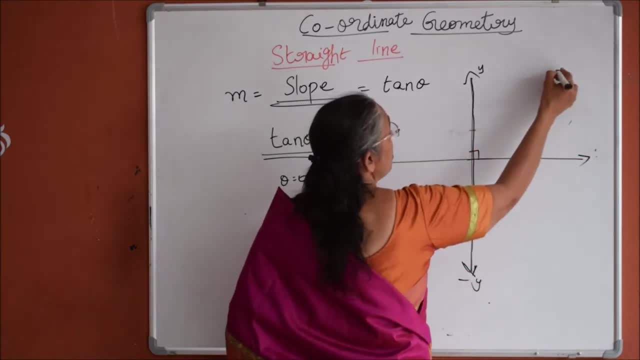 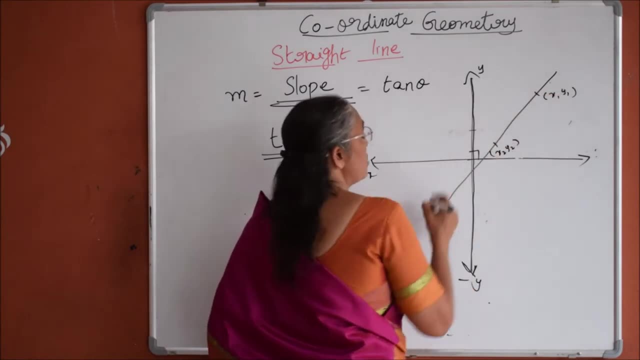 is a line joining the two points. Okay, Two points on the line is given, So here x1, y1 and this point is x2, y2.. Angle is not given, But we know tan theta is slope, But we want. 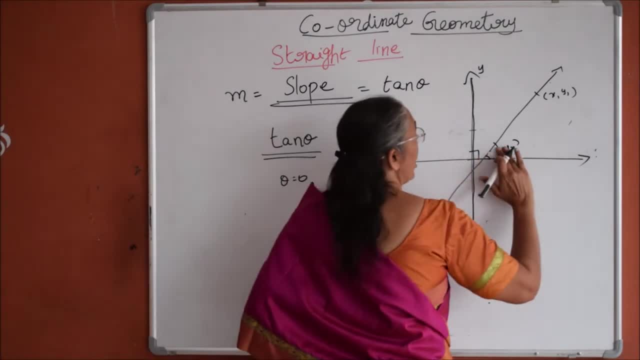 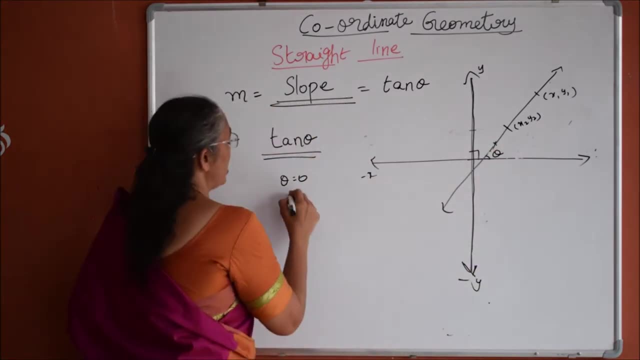 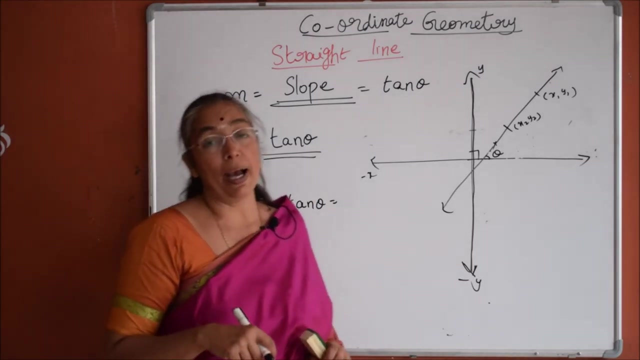 to find the slope of this line. So how can we find? Okay, let me take this point- x2, y2 here. Okay, So this is theta. So what is our tan theta? We discussed what is slope of x axis- slope of the line parallel to x axis. slope of y axis: slope of the line parallel. 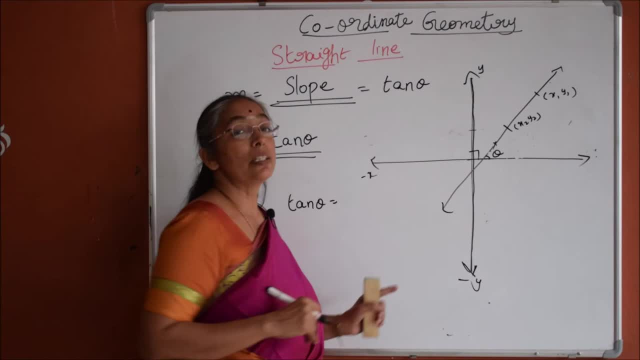 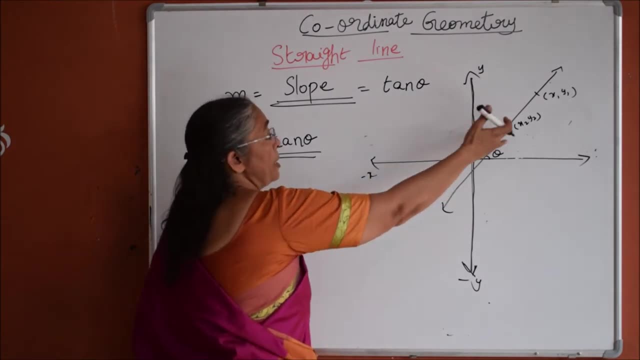 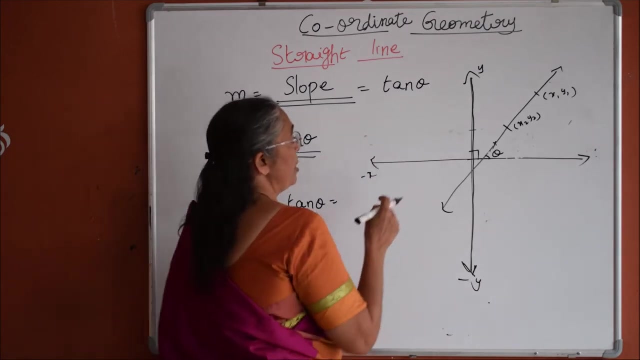 to y axis. Now, apart from that, now general line, this line is making an inclination of theta. So tan theta is our slope. But how to get the slope in terms of x1, y1 and x2, y2? So our tan theta is slope. Yeah, Now I want slope in terms of x1, y1 and x2, y2, which 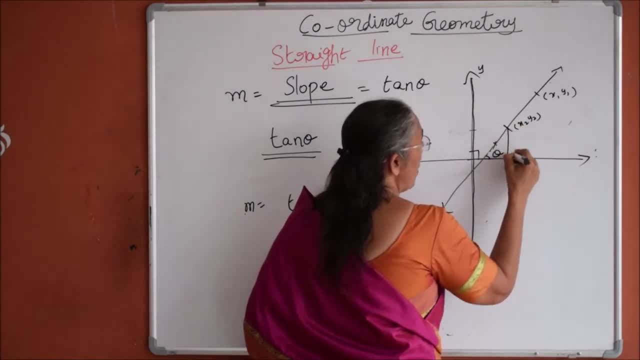 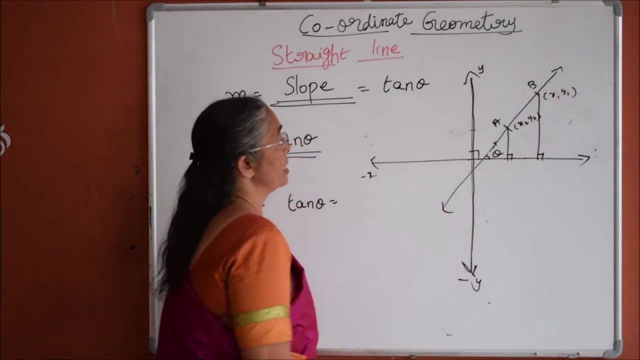 are the points on that line? Let me drop a perpendicular from. let the point be a and b And drop the perpendiculars from a: x1, a I consider as x2, y2.. Okay, Or a, we will consider as x. any way, we can consider x2, y2, and b is x1, y1.. Now here, drop perpendicular from. 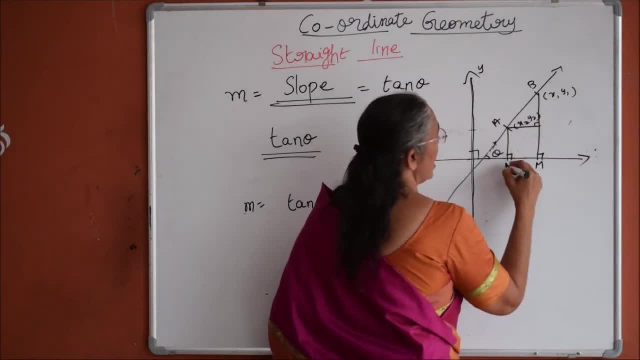 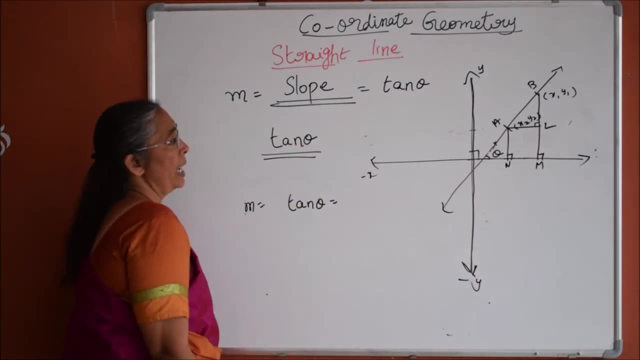 the point a on this is suppose m n bm. I will make this one as a l. Okay, Now triangle a, l b is right angle triangle for us. Okay, Fine, We need only tan theta. Okay, Now we go here. this is see this line and these two lines. 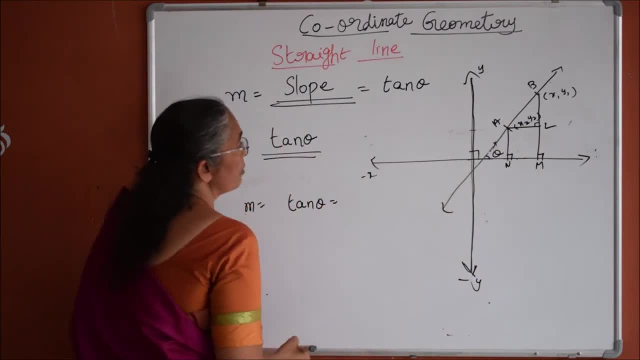 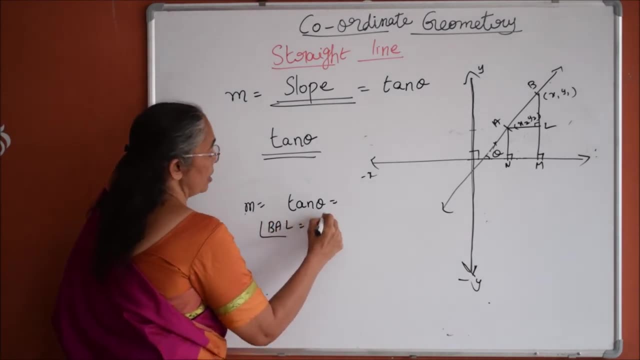 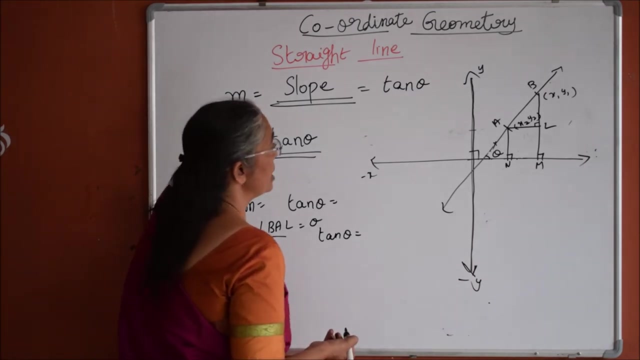 are parallel, So corresponding angles are equal. So angle b a l, angle b a- l is theta. So tan theta is equals to what is tan theta is equals to Opposite side by adjacent side. So opposite side is, for this is the right angle for you. 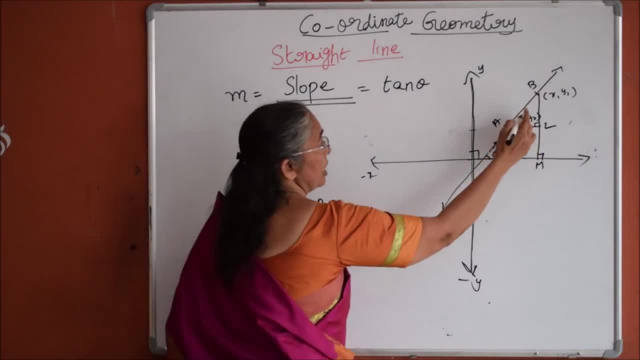 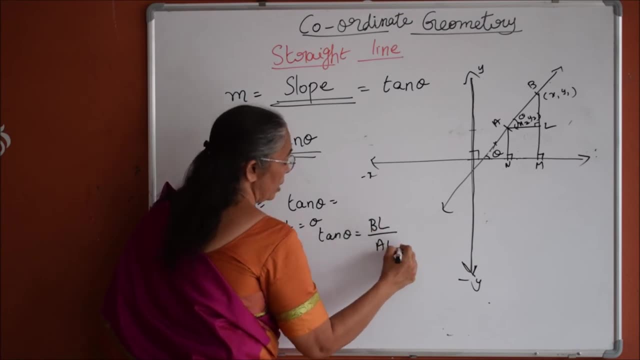 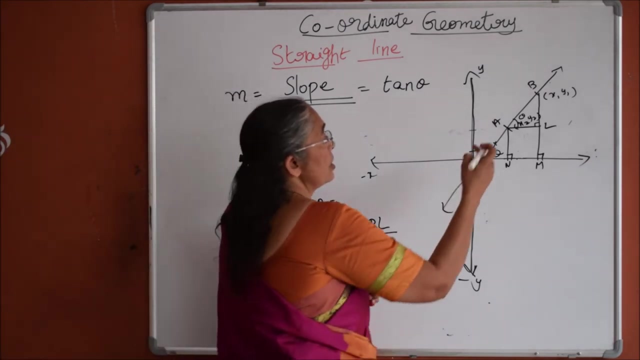 this is right angle and here a hypotenuse: So tan theta, this is theta. So tan theta is equals to opposite side. is BL, BL divided by AL. Now, what is BL? From the points we marked? BL is nothing, but see this is this distance we need. BL is BM minus LM. BL is 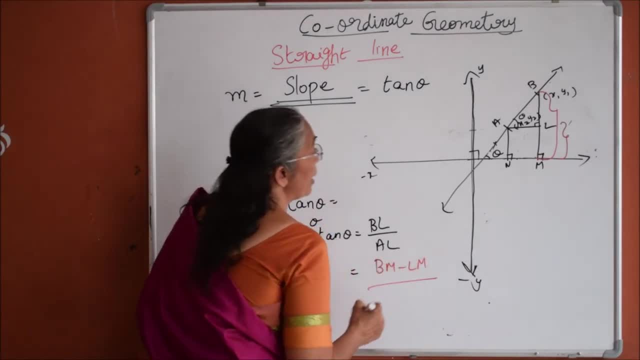 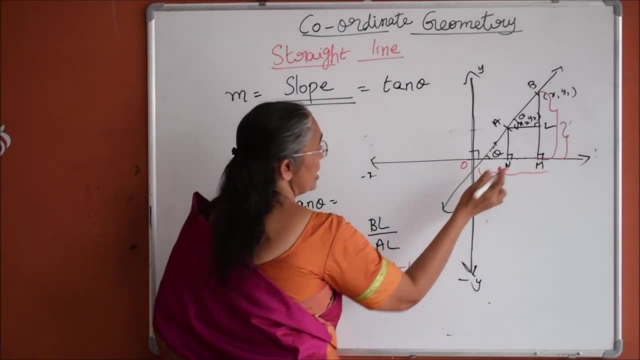 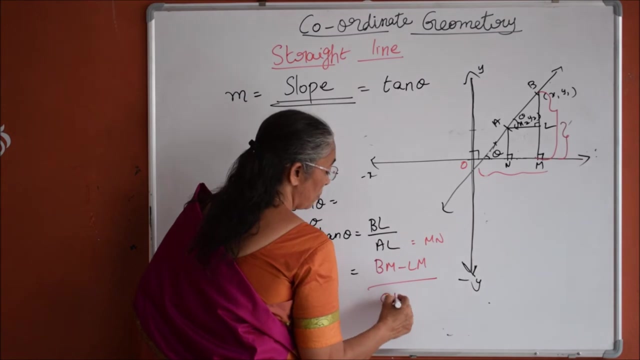 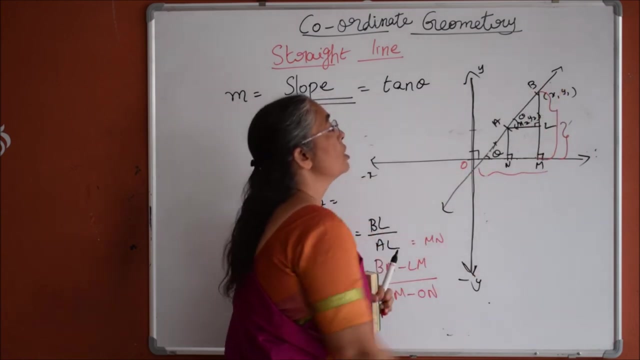 BM minus LM divided by AL. AL is suppose origin. this is OM. full distance minus AL is same as MN first, which is equal to MN. How can we write MN, OM minus ON? Okay, Fine, So what is your BM now? BM is this whole distance, So that distance is nothing but Y1.. So Y1.